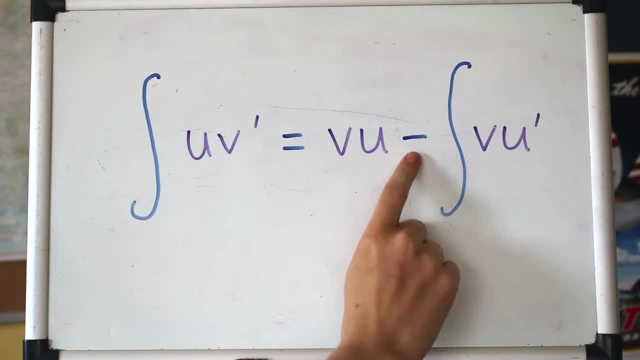 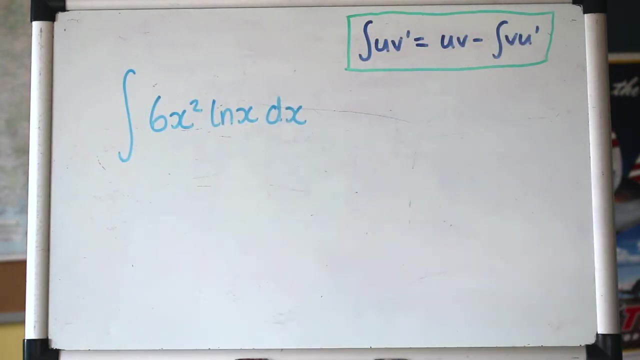 u and v, multiplying them together and taking away the integral of them, the opposite way around. So v times the derivative of u. Let's work that through with some examples. Okay, here we've got the first question and I've just put the formula up in the top right corner, just so we can remember it. So here's the first example. 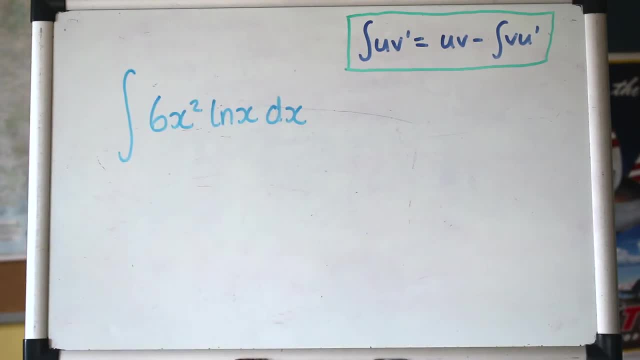 So if you're trying to take something multiplied by v bar, you might be told to look at the u, because v is the newun, and when there's newu and v bar but not v bar, you could take the other two, so v dash and v prime. So then you might notice that it looks horrendous. 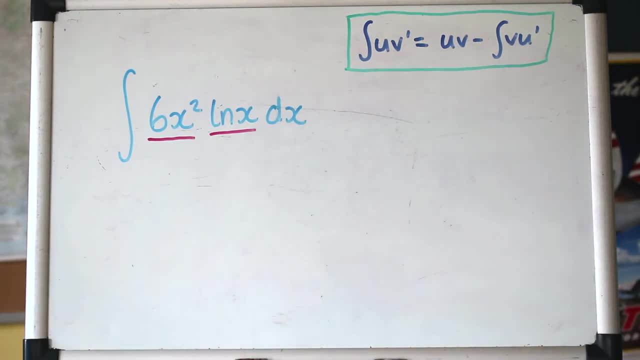 There's no other way to integrate this, really the other methods. if you tried them you wouldn't get very far. But here we've got 6x squared being multiplied by ln x. There's two things being multiplied together. so already it looks a bit like that, But we just need to decide which one's going to be the u and which one's going to be the v dash, Which one of them would be helpful to treat as already being differentiated. 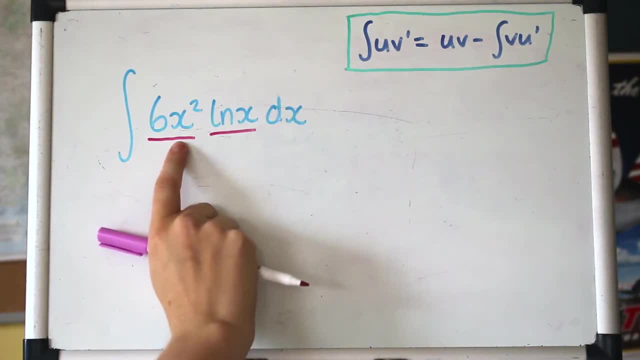 x squared. we can either differentiate or integrate, so that one is pretty flexible. but log of x, you can't actually integrate that very easily. In actual fact, you can integrate log of x and I'll show you how in this video actually, but it's not easy. 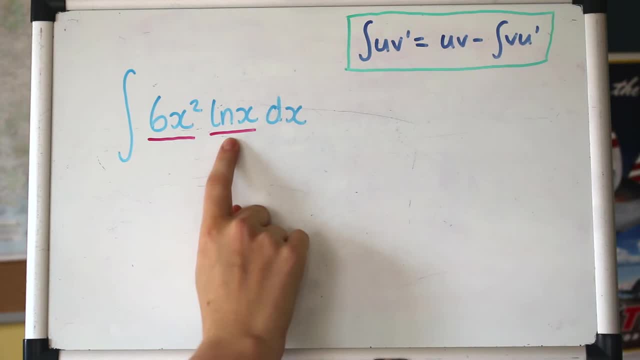 so it's a good idea, instead of integrating that, to differentiate it. So we're going to treat that as our u, because then we can differentiate it to get u dash, and that means that this one can be our v dash. So what I do is write. 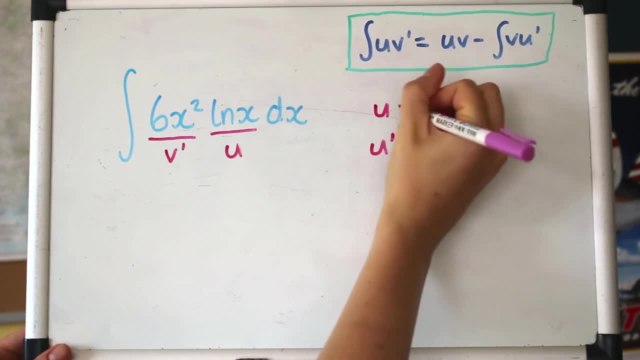 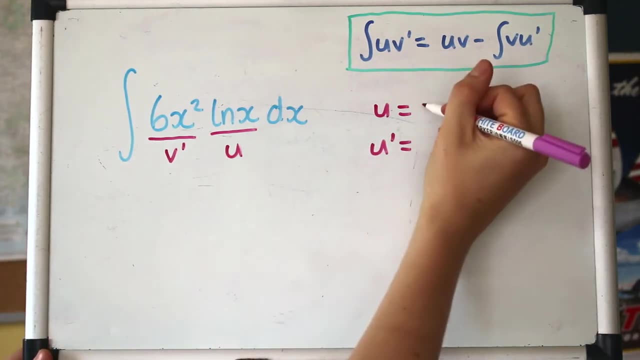 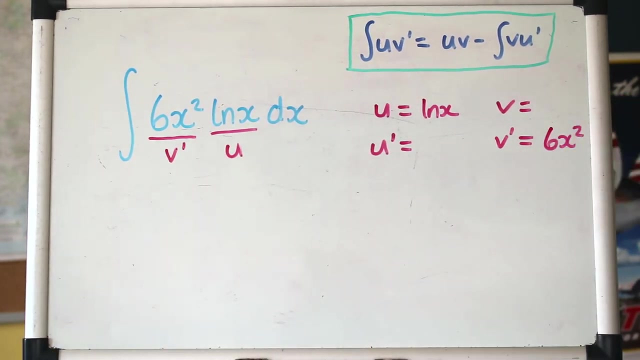 to the side u and u dash and v and v dash. So we've decided to make u log of x, meaning that v dash is the 6x squared. Now we need to fill in the rest of the information. so we want u dash, which means we differentiate that and hopefully you know. 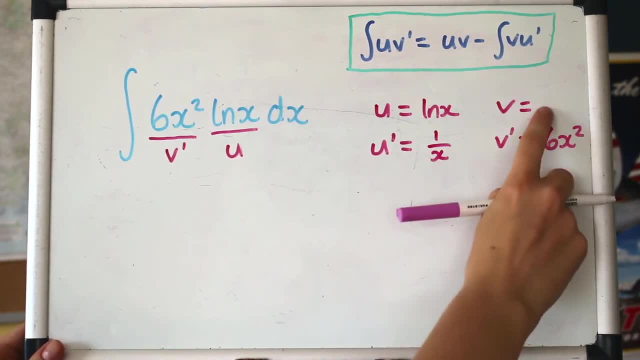 that's 1 over x. Now we want v, so we've already got the derivative 6x squared. we want to go the opposite way. we want to integrate that, So that's a straightforward integration. hopefully you can do that without too much problem. 2x cubed. 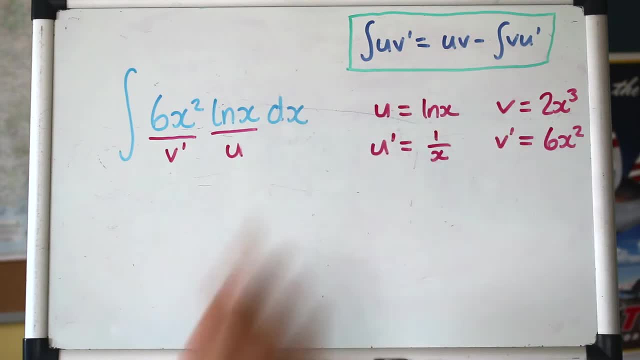 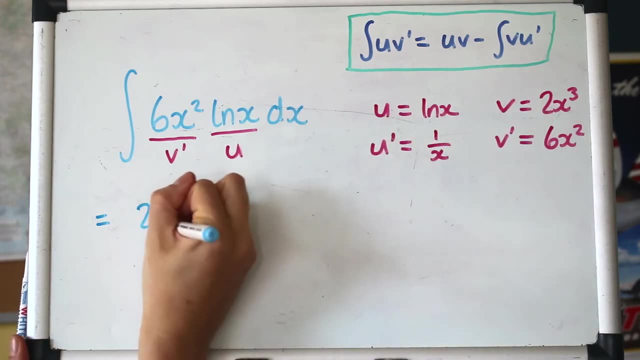 Now that we've filled in those pieces, we're just putting them into the formula. So we've got u times v. that's log of x times 2x cubed. I'm going to write the 2x cubed first, just because that's convention. 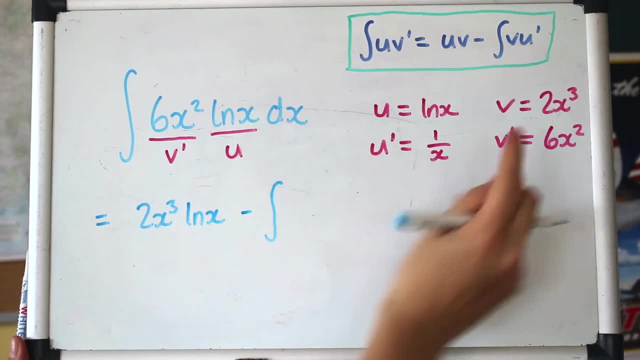 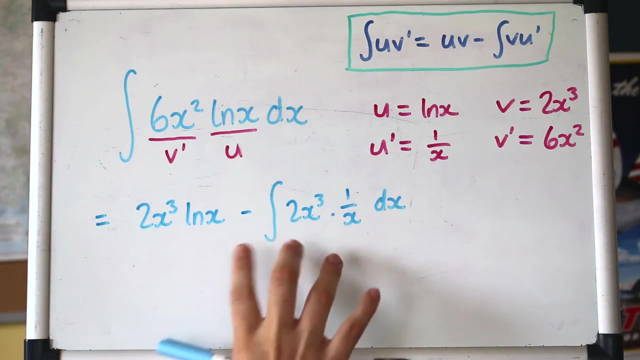 and then minus the integral of VU dash, so 2x cubed times. I'll just put a dot for times 1 over x with respect to x. So the idea behind integration by parts is to force it into a form where what you've got left to integrate should be okay. 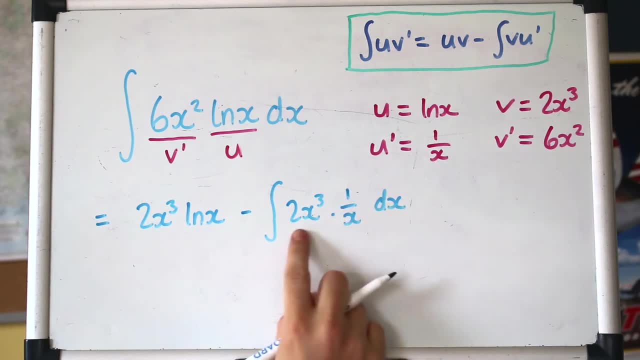 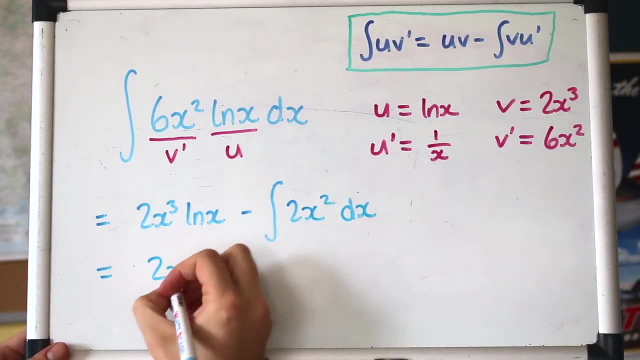 So we can simplify this. first We're dividing by x, so we can simplify that to 2x squared, And so that stays the same at the front, And now we want to integrate that Again. it should be a straightforward integration. 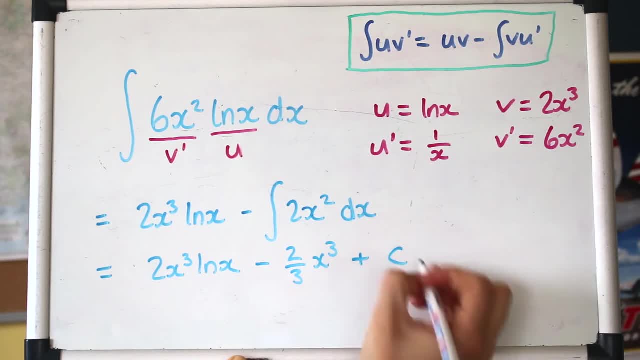 And because this is indefinite, there are no limits- we need the plus C. Great hope, that's clear. If you need to rewind and have a go at that yourself, please do, Otherwise we'll do another example. Okay, second example. 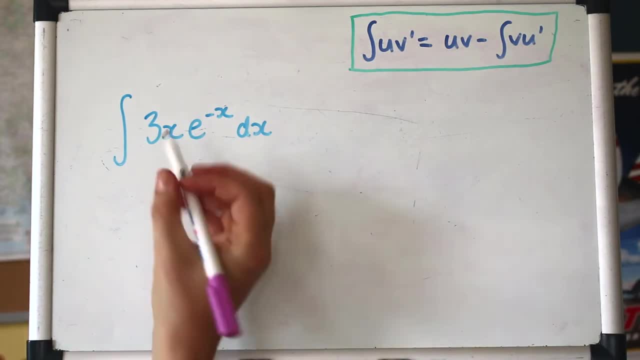 So here again we've got something that looks really difficult to integrate, but we've got two things that are multiplying together This time, both of them you could differentiate or integrate, so it's not like the last one where it's quite so obvious which one to make which. 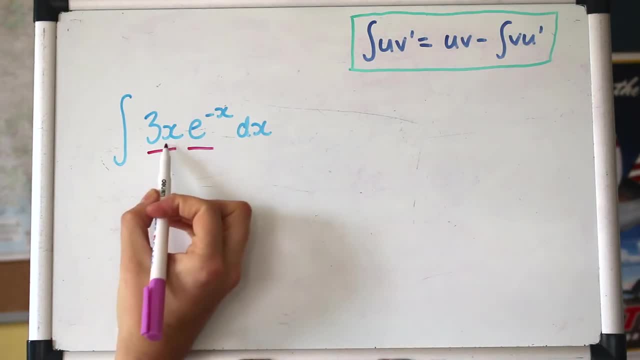 But notice the 3x here. If you differentiate that, you would just be left with 3. And that would get rid of an x, and that's a really helpful thing, because then what you'd be left to integrate would be much easier. 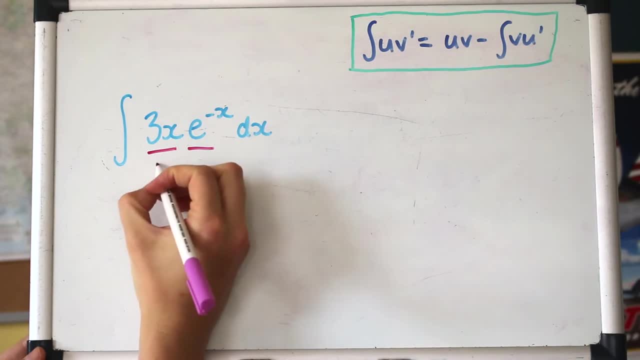 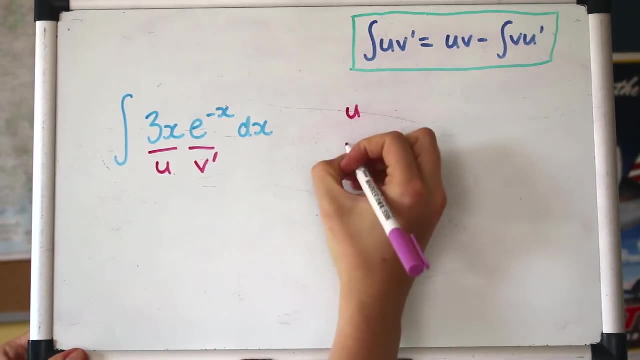 So we're going to differentiate that one, which means we're going to make that U And then that one will have a plus And that one will have to be V dash. Okay, so let's put in the information and hopefully that will be clearer. 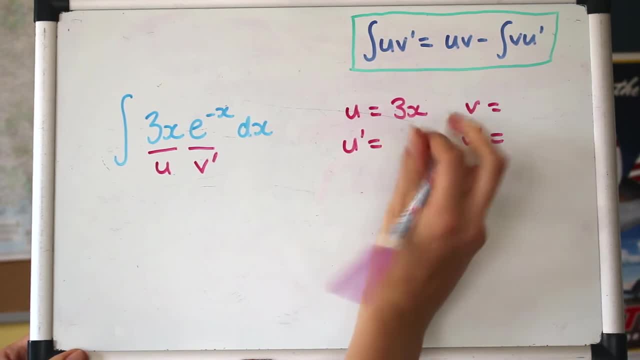 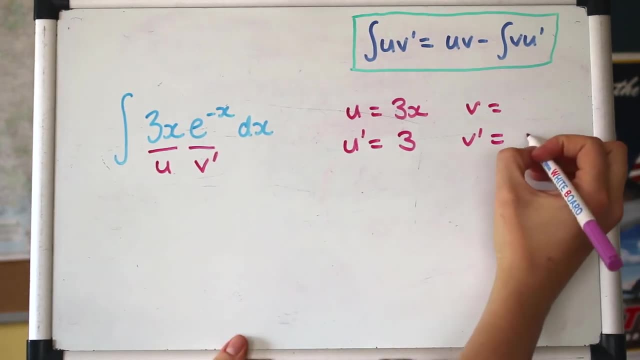 So we're saying that 3x is our U, and that means that we can differentiate it. So we're left with just 3, and that's a really nice thing to do. V dash then will be e to the minus x. 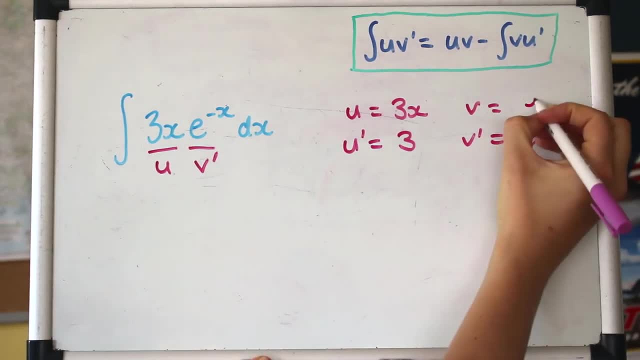 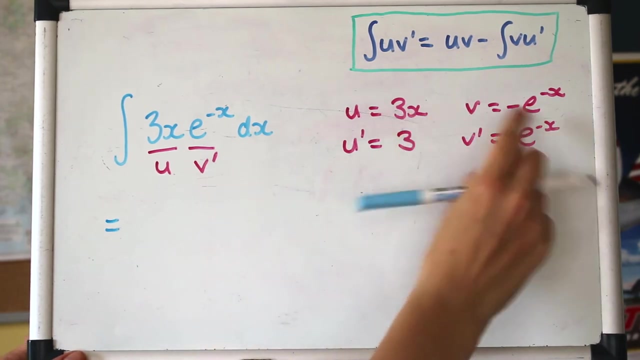 And integrating that backwards. so we'll have e to the minus x and divide by the derivative of minus x, which is minus 1.. So it will be minus e to the minus ex. Okay, then, putting that into the formula. So U times V, we've got these ones multiplied together. 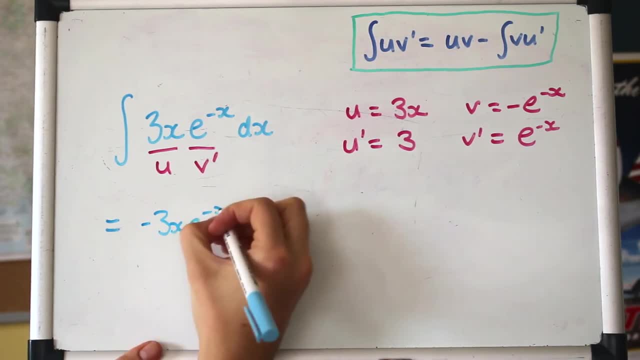 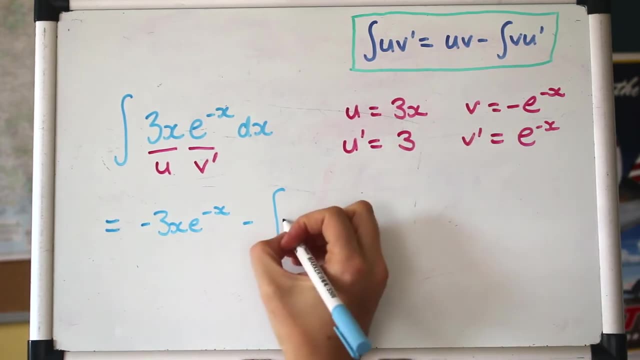 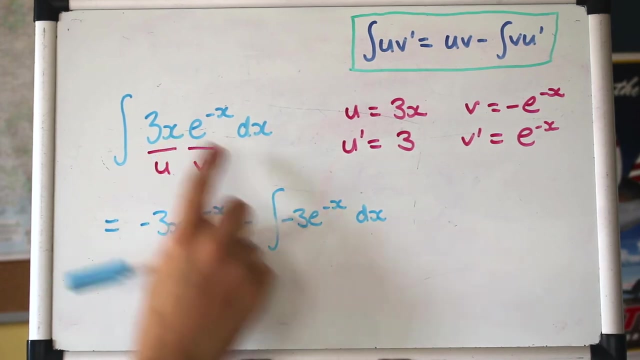 I'm going to put the minus at the front, 3x e to the minus x, Okay, and then we're taking away the integral of V U dash, So these ones multiplied together. So can you see what I mean? Now we're integrating something where we've dropped the x. 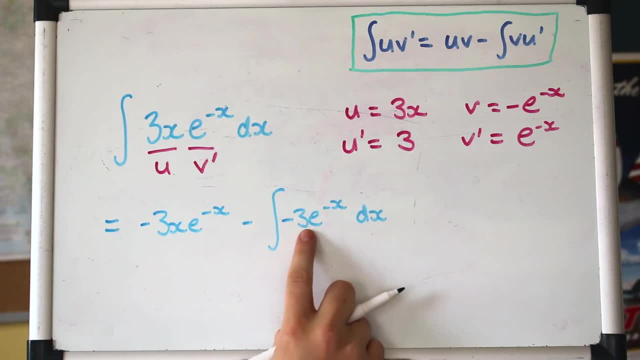 So getting rid of that x, So getting rid of that x by differentiating, is a really good thing, because now that is much easier to integrate directly. Just to make it easier, I'm going to pull the minus into the front before I integrate that, just so we don't make any mistakes with the signs. 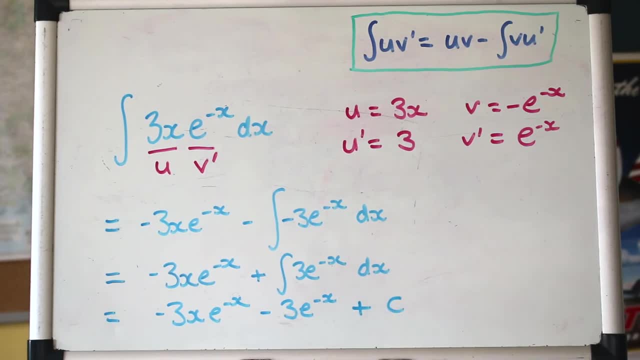 And we need the plus c. Great, well done. if you're getting that. Differentiating and integrating e to the x or e to a function is in one of my other, I think- differentiation videos, So if you're not sure about that, do check that out. 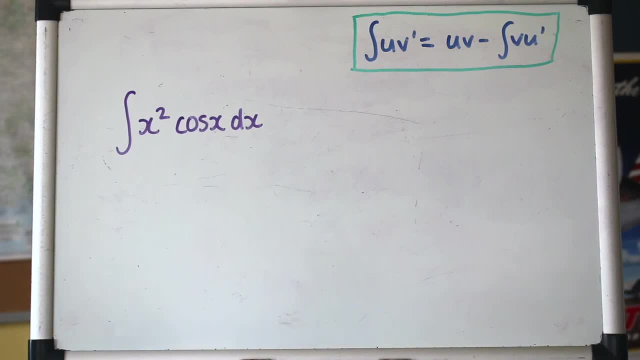 Okay. third example is a juicy one. Trig always makes things interesting, doesn't it? So, trying to decide which way round to make these U and V dash x squared, if you differentiate it, well, if you differentiate it twice, 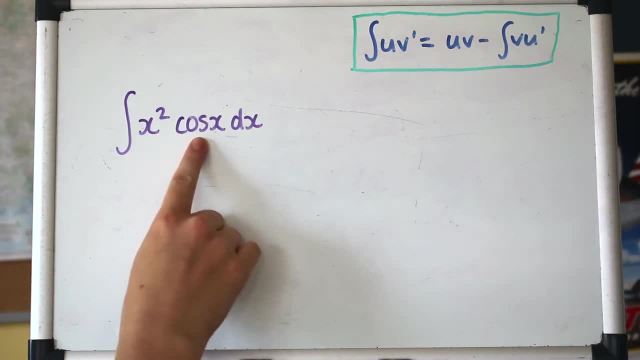 you'll get rid of the x Cos when you differentiate. it'll just alternate between sin and cos when you differentiate and integrate. So that's not really going to change an awful lot. So it's best to differentiate that one. So we'll make that U and we'll make this one V dash. 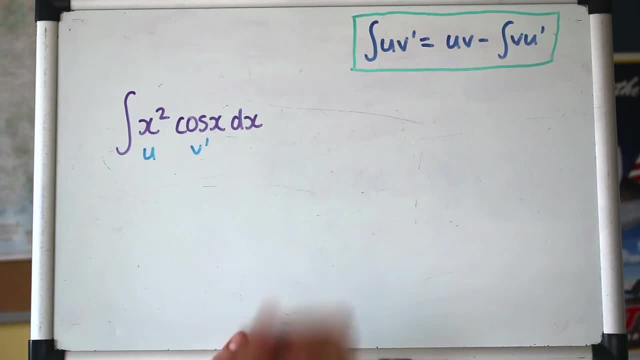 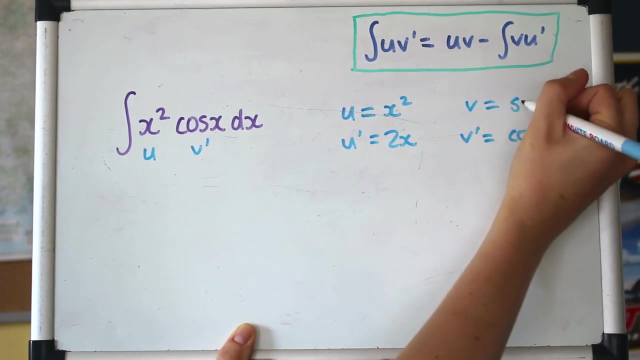 And what is going to happen? Well, actually I won't tell you yet. We'll find out. So U is x squared. Differentiate that to get 2x V. dash is cos And we need to integrate that back to get sin. 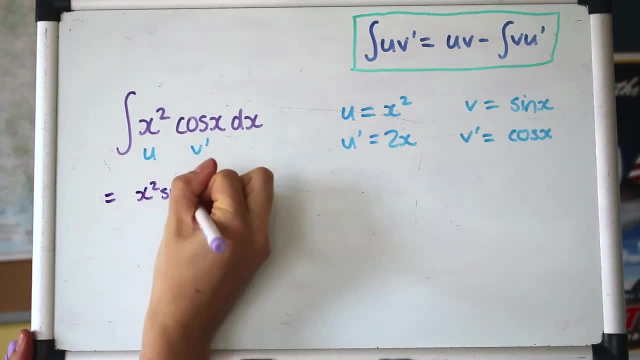 Using the formula U times V minus the integral of V. U dash. A lot of the time with maths you're just trying stuff and playing with it and seeing what works. So if you weren't sure, if you could just try that and then see what happens. 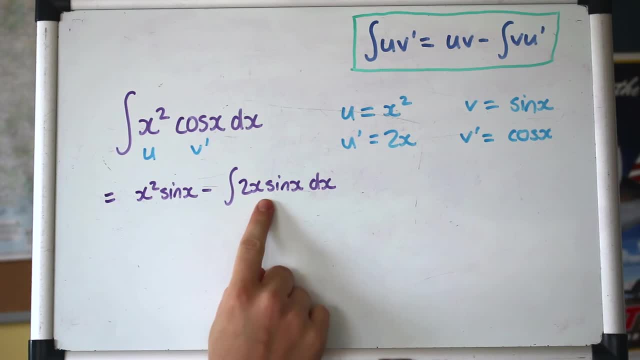 Let's see what we've got. Notice that this integral here it looks easier to integrate than this did, But we're still not quite in a position we can integrate it because we've still got an x, So that one we had x squared. 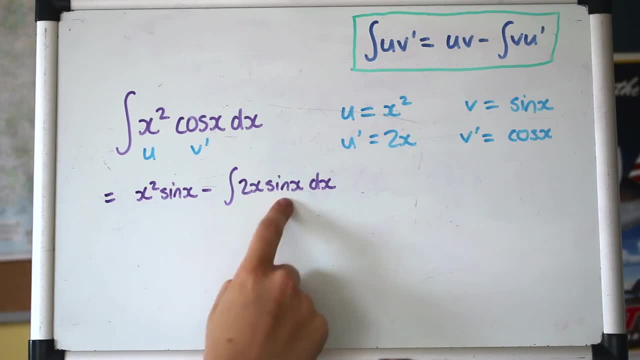 This one. we've got x, So we're a step closer. What we really want is just a number times sin x to be able to integrate that. So what we're going to do is use integration by parts again. We're going to apply it again to this part here. 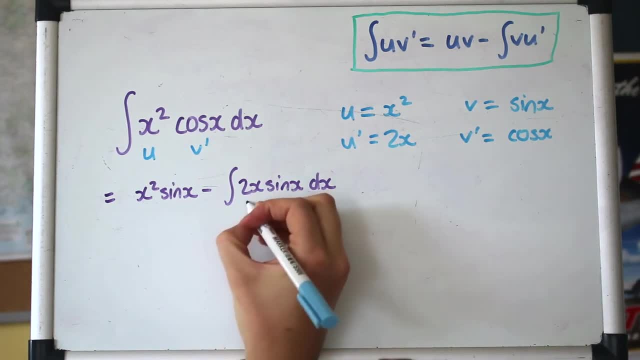 Fun times. So if we make the 2x U and the sin x V dash, then when we differentiate 2x we'll lose the x. You can actually use integration by parts as many times as you want. Just have a great time. 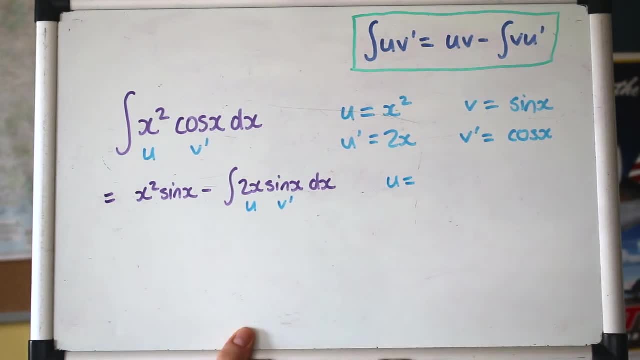 But generally in A level. you'll only be expected to do it up to a maximum of two times, hopefully. So let's make that 2x and U dash then will be 2.. V dash now is sin x And just being really careful about the negative sign. 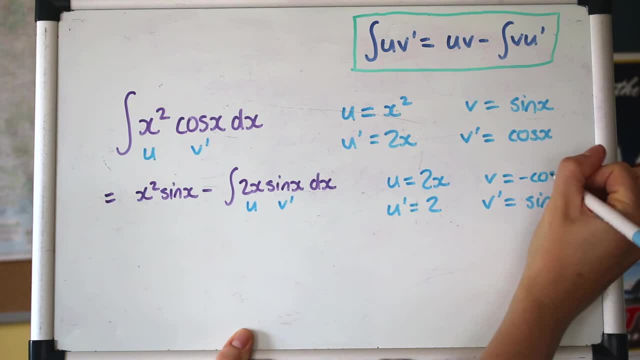 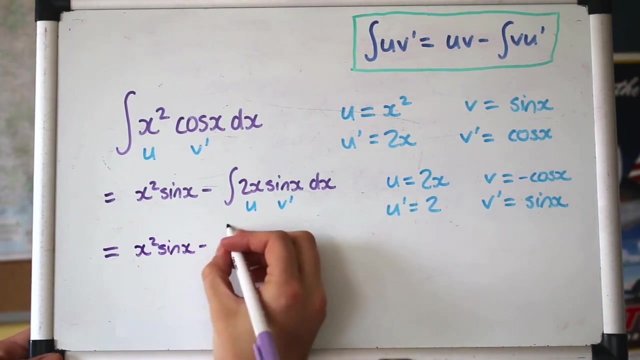 When you integrate that back, you'll get a negative cos, Because when you differentiate cos it changes the sign Sine of sine. Okay, So we've still got that beginning bit there, x squared sin x, And I'm going to put minus and then all of this in brackets. 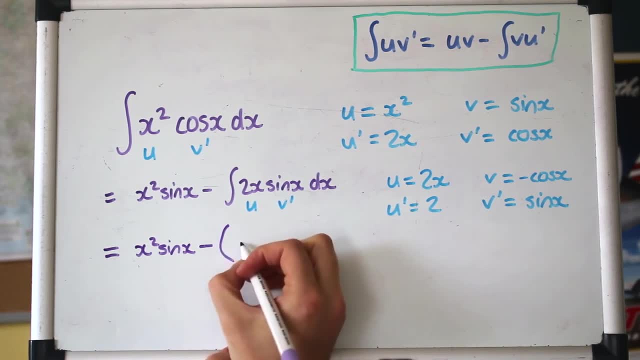 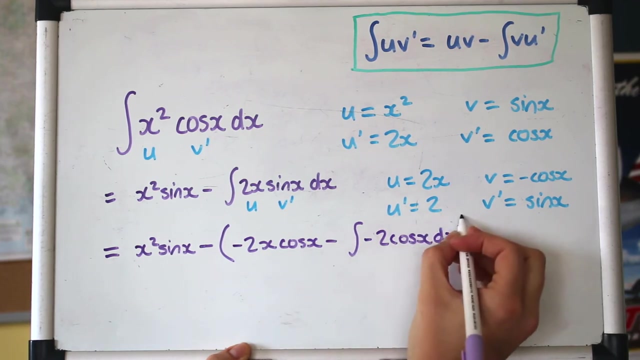 because that minus needs to apply to all of it. So let's now use the integration by parts formula again. So U V will be minus 2x, cos x, Minus 2x, That's the integral of that stuff there. Now we can integrate that directly. 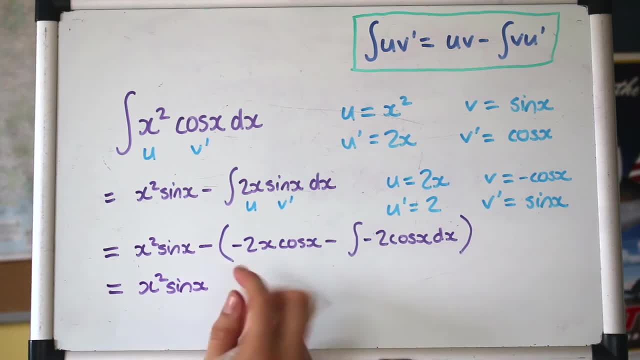 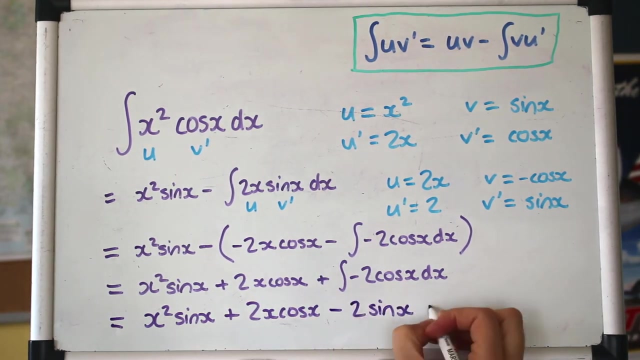 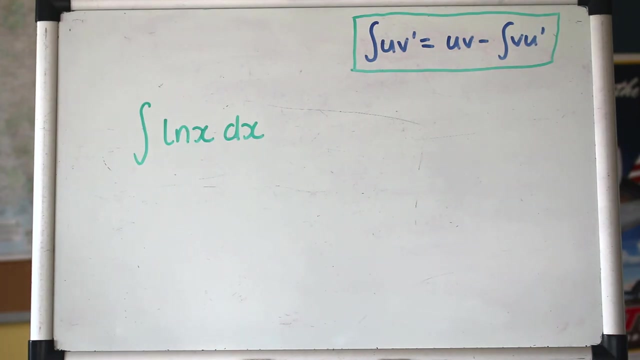 So still with this stuff here, I'll remove the brackets now and change that to a plus And integrating that we'll get minus sine x. Let's see, Okay. third example: I said I'd show you how to integrate log. 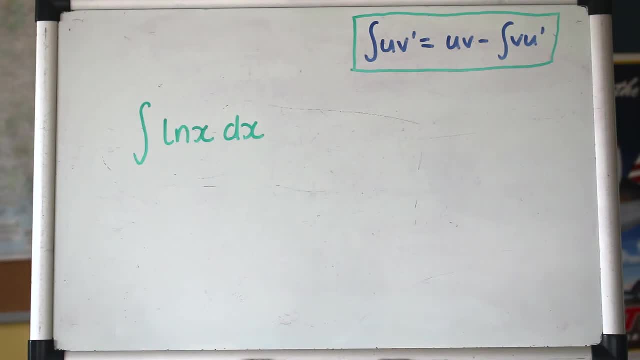 I like this because it's just really clever. So this is a trick you can pull if you are faced with something that you can't really integrate. So log of x. it doesn't have a straightforward integral. It feels like something you can't integrate. 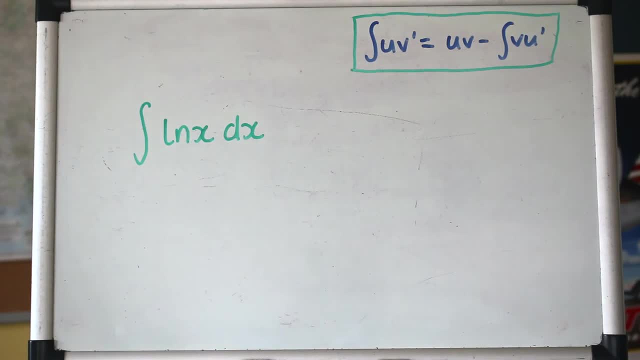 But you can, using integration by parts as a clever trick. So what we're going to do is sneak in 1 times log of x And then, because you can't integrate log of x easily directly, we're going to instead differentiate it by calling it U. 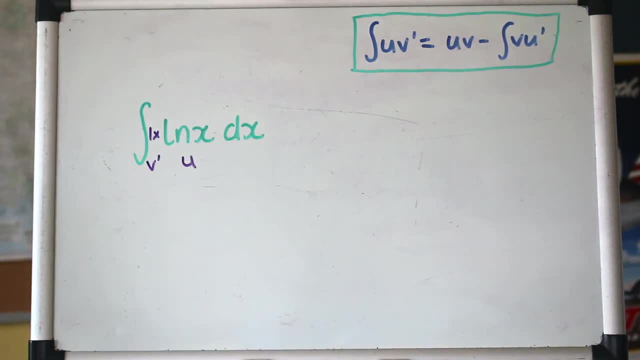 And then the 1 will be the V dash. Isn't that sneaky? So then we're integrating log of x to get 1 over x, And the V dash is 1.. Integrating that back, we just get x. Now we can use the formula. 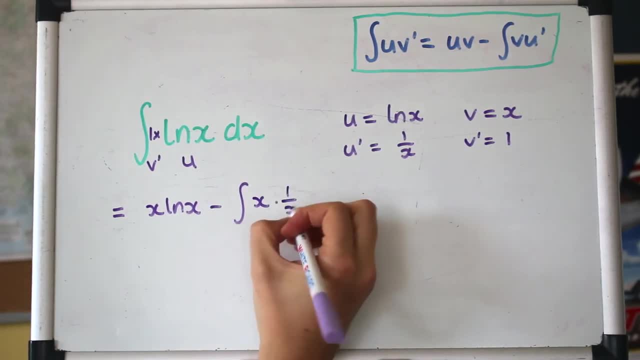 So we've got x times 1 over x, which of course is just 1.. And integral of 1 is x. Beautiful, Some people just learn that that's the integral of log of x, But I think that's so fun. 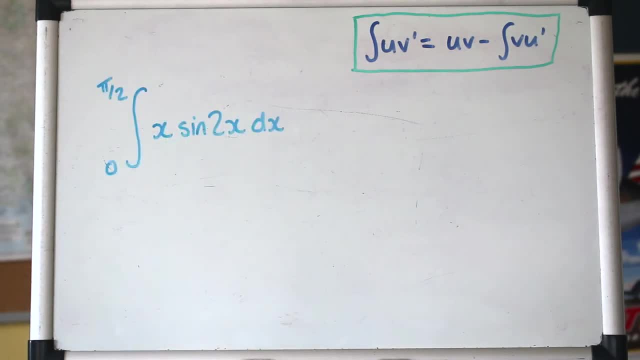 You should just do it yourself. Okay, always practicing more trick, And this time we're going to have limits, So I'll show you how. I'll show you how to use them in the integration by parts, using definite integration. So same thing to start with. 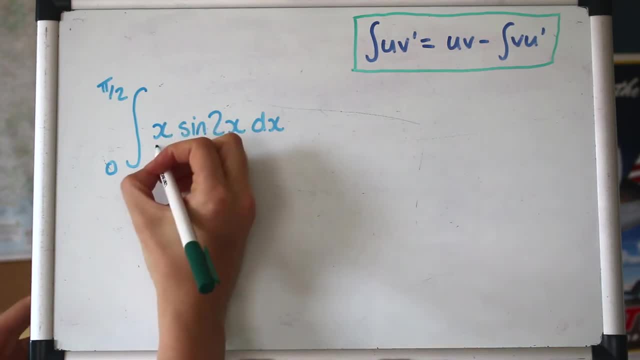 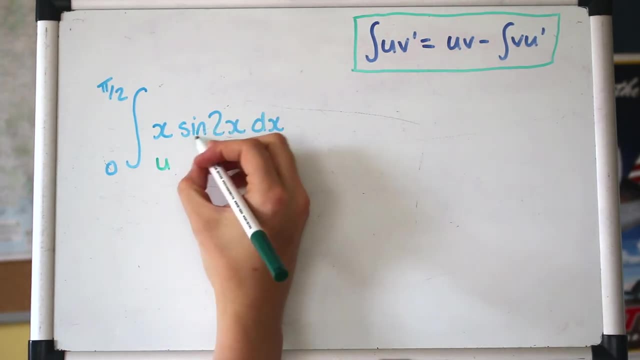 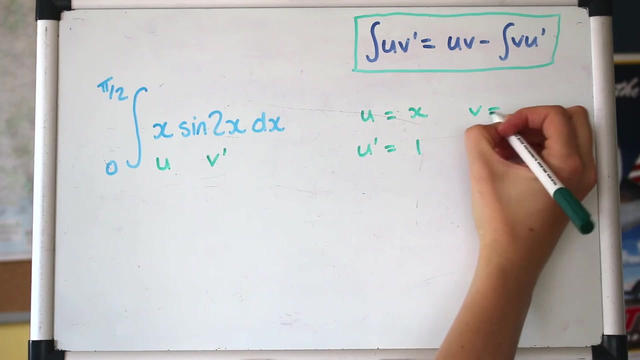 We're going to label it up with U and V dash. Here the x will make that U, because if you differentiate it you'll just get 1.. So you drop the x. That's really handy, as we know, And that means that sine of 2x is our V dash. 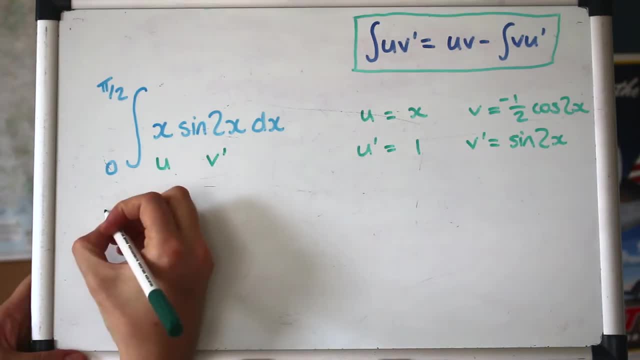 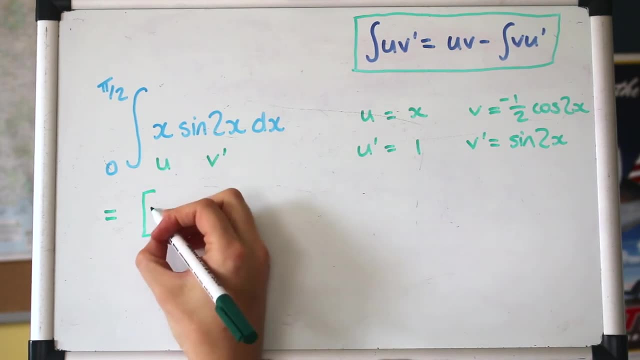 Just snuck in a minus there, Don't forget that. Okay, using the formula. So the first bit, the UV. I'm going to put that in the square brackets because that doesn't need integrating again now. It's already sort of been integrated. 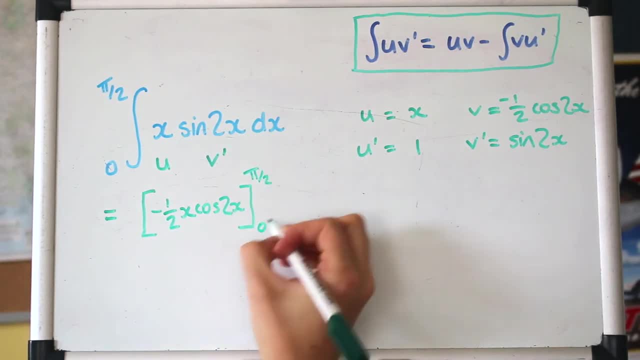 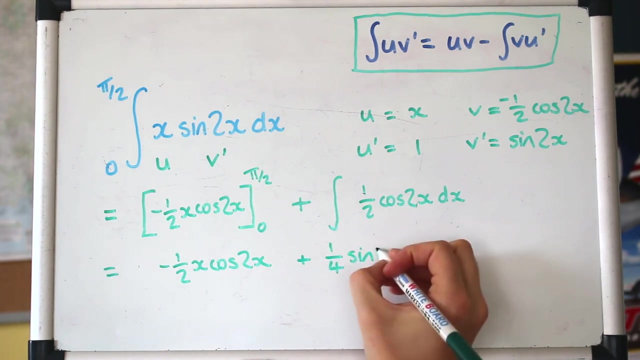 So putting the limits on the end. I've got a minus and a minus here, so I'm going to pull that out and make it a blur Integral of that there And now, because it's all been integrated, I can put the whole lot in the square brackets. 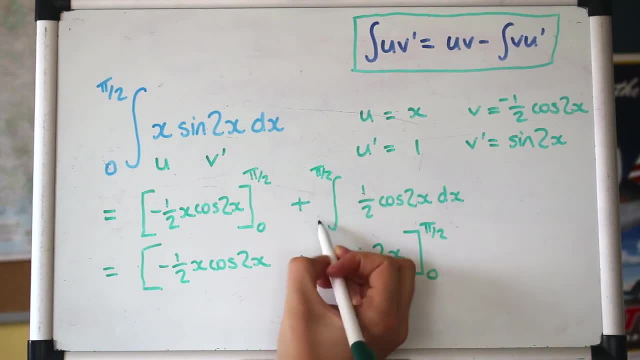 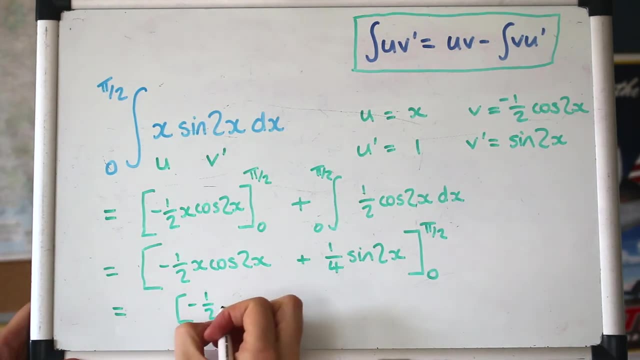 I should really have written the limits on here as well. It's just a lot of writing, isn't it? Good Now we can do one minus the other, So cos of 2, lots of pi over 2 will be cos of pi. 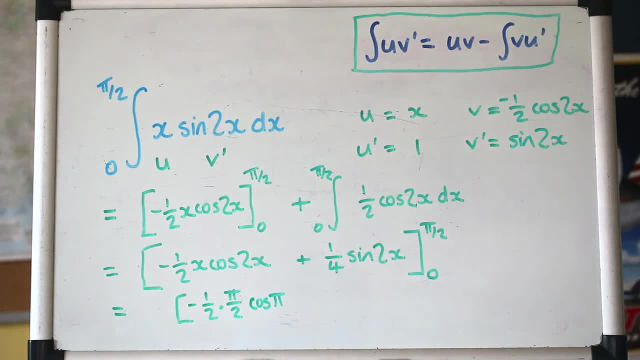 Hopefully you know that without using a calculator And when we put pi over 2 into here, we'll have sine of pi. Hopefully you know that's 0. Now putting 0 into all of this, we'll have half times 0,. 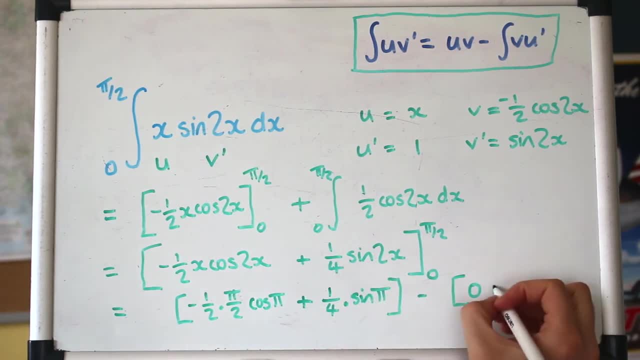 so that's just 0. And there's plus a quarter sine of 0, and a sine of 0 is 0. Lots of 0s going on. Sine of pi is 0. Love it when that happens. So we're just left with this here. 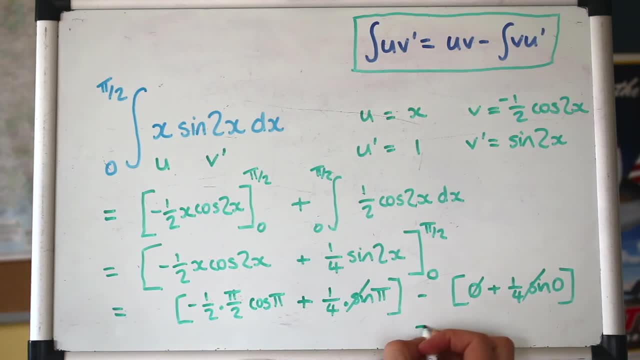 Cos of pi is minus 1. So that will times with the minus at the front, so we'll get a positive quarter pi or pi over 4.. Nice, And that was actually pulled out of a past exam paper, so that gives you an idea of the standard. 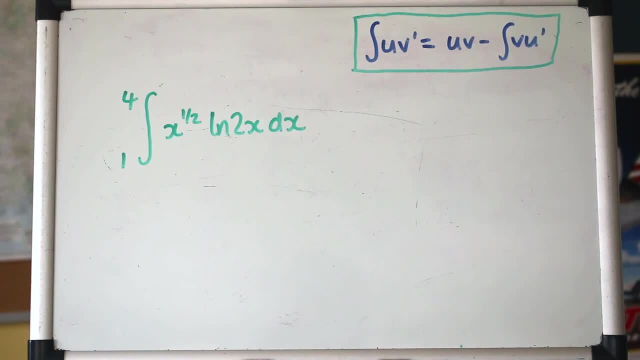 Let's do one more question to finish. OK, last one. Have a go at as much of this as you can yourself. I'm going to make the log of 2x. I'm going to make that the? u cos, as we know, it's not very easy to directly integrate. 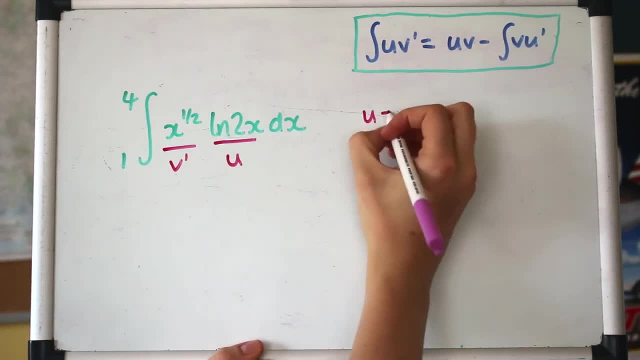 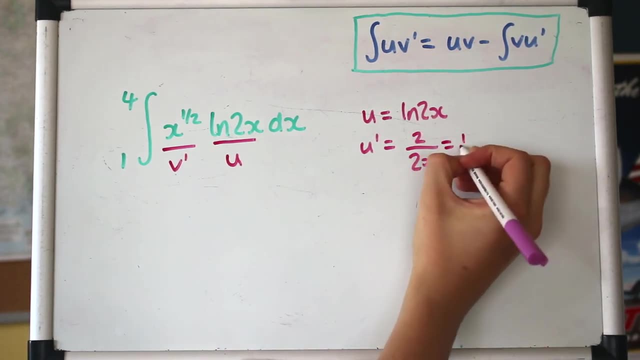 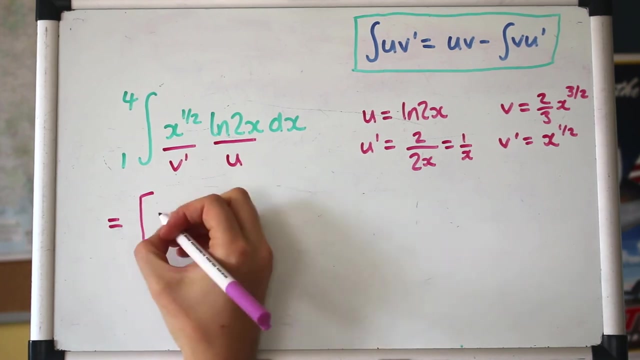 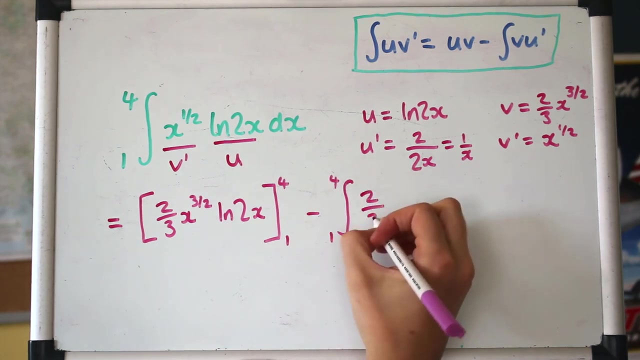 The x to the half can be the v dash. So when you differentiate this you'll get 2 over 2x. so that's just 1 over x. Integrating Here I've multiplied the v and the u dash together. 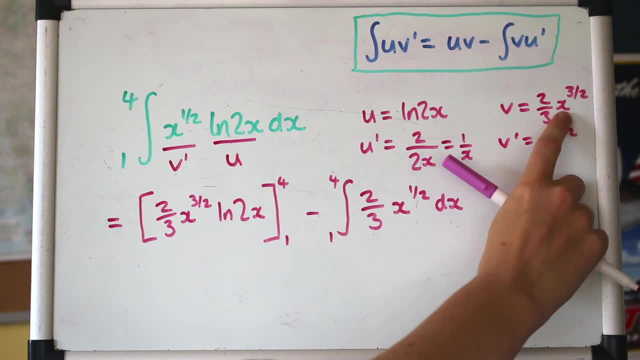 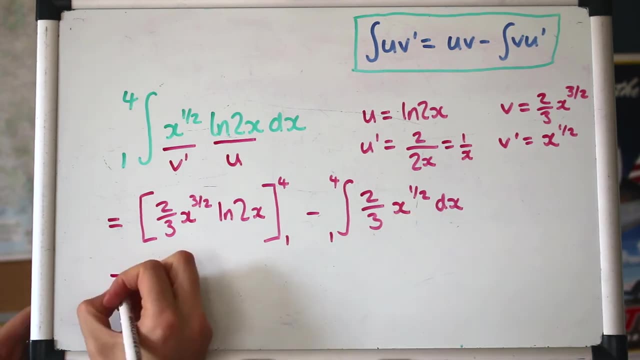 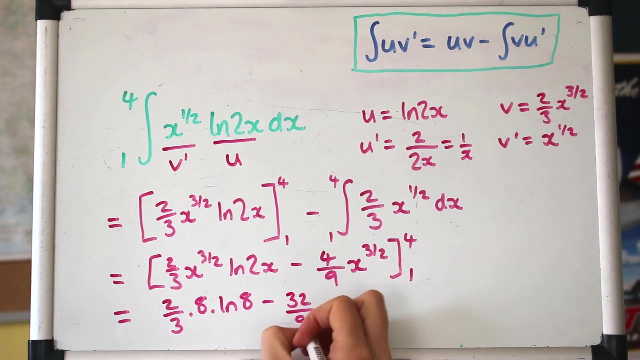 and the u dash is 1 over x, so I've just divided by x. So that's taking 1 off the 3 over 2 to leave just a half in the power. OK, putting in the limits, Totally run out of room. 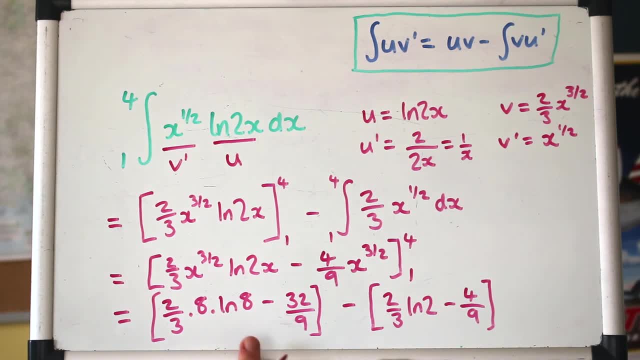 so I'm just going to have to change it on this line. but anyway, We've got log of 2 here. We want to clean up and collect stuff together, Log of 2 and log of 8.. But notice, you can write log of 8.